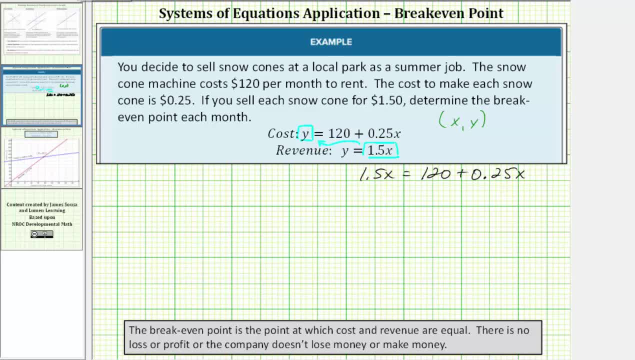 let's get the x terms on one side of the equation. So to undo plus 0.25x, we'll subtract 0.25x on both sides. And now we simplify: 1.5x minus 0.25x is 1.25x. 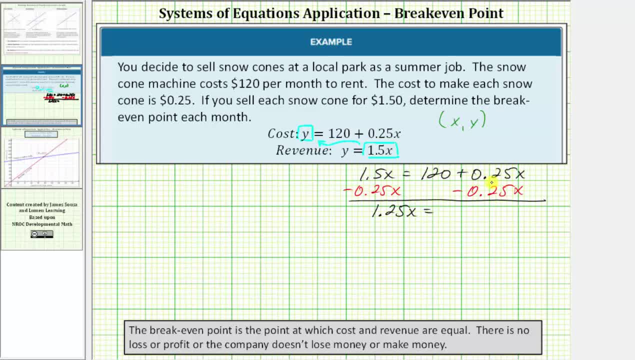 So we have 1.25x equals on the right plus 0.25x. So 0.25x minus 0.25x is 0.. So the right side simplifies to 120.. And now to solve for x, we divide both sides by 1.25.. 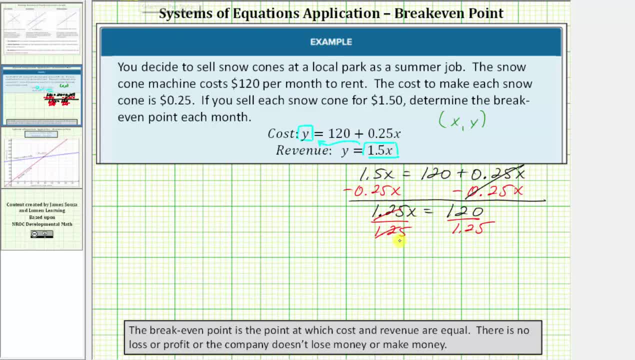 Simplifying this quotient is one: One times x is x. So we have: x equals 120. divided by 1.25 equals 96. So now we know for the break-even point, the x value is 96.. You still need to find the y value. 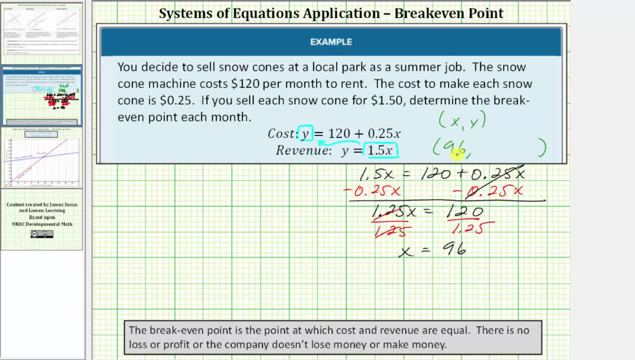 But because we know the x value is 96,, this means you must sell 96 snow cones each month in order to break even. And when x equals 96, both the cost and revenue should be the same or should be equal. And let's go ahead and verify this. 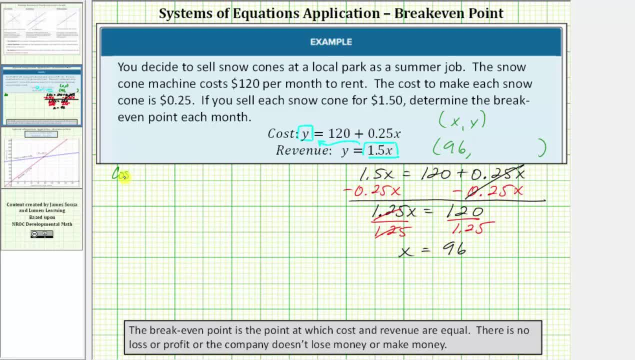 Let's first check the cost when x equals 96. The cost would be: y equals 120 plus 0.25 times 96. Which would be 120 plus 0.25 times 96 is 24.. And therefore we have a cost of $144 when x equals 96.. 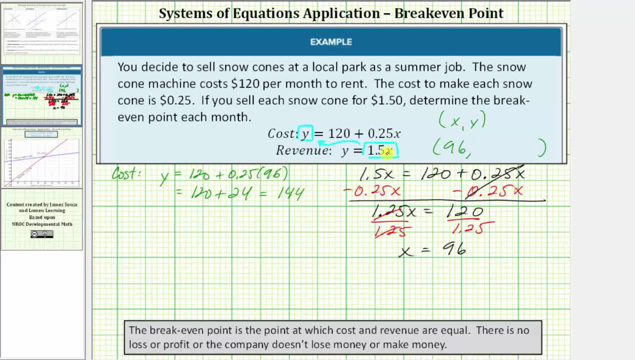 Now we should get the same amount for the revenue when x equals 96.. Again, let's go ahead and check this. Revenue is y equals 1.5 times 96, which is equal to 144.. So now we know the break-even point is 96 comma 144.. 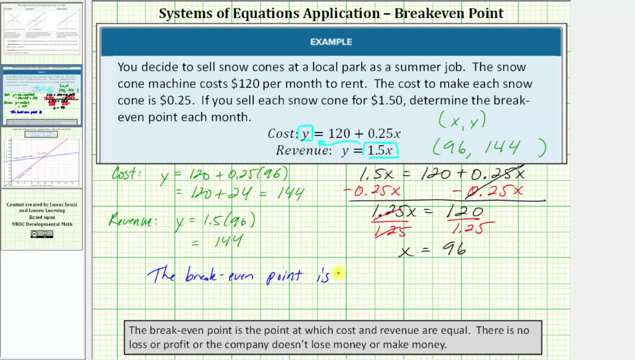 Let's write this as a sentence. The break-even point is 96 comma 144,, which means if you sell 96 snow cones per month, you won't lose money or make money, Which means if you sell more than 96 snow cones.